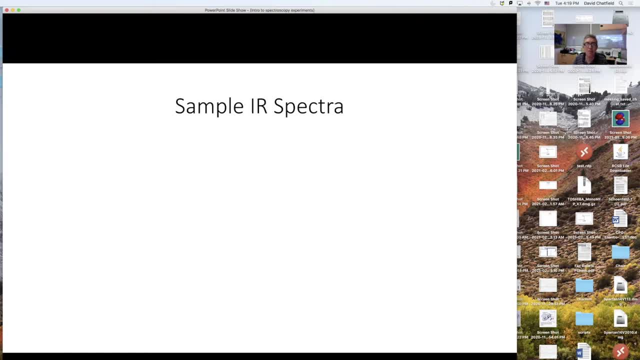 cell. This is a brief picture of the spectrometer. So first a couple of pictures of sample ion spectra. You may be used to pictures like the one on the left from organic chemistry. that is often a solid or liquid state sample. It's very broad. It's not highly resolved. 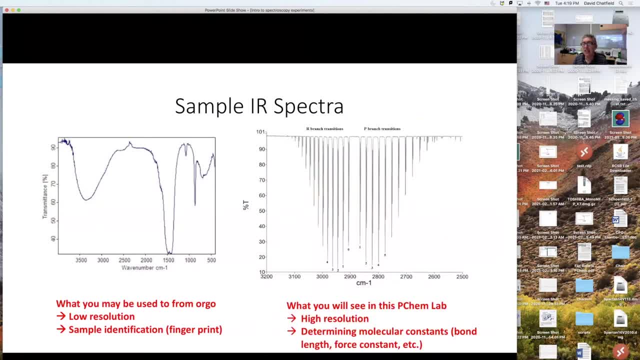 It's useful for sample identification, kind of like a fingerprint. We are going to have in this lab much more highly resolved spectra where we can see the individual peaks. They're highly resolved for a couple of years And there's a couple of reasons. One is their gas phase, not condensed phase. Another is 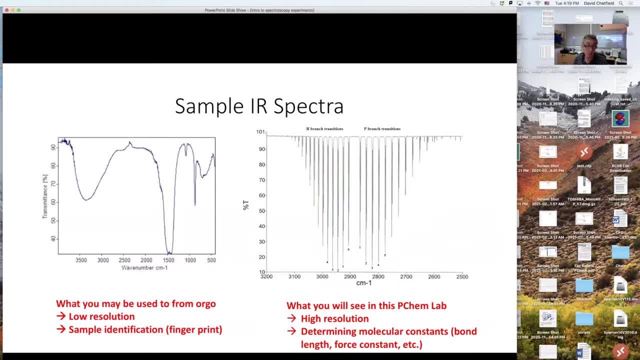 that HCl, it's a diatomic. It's a fairly simple thing And we have a very highly resolved, very powerful spectrometer, So we'll interpret this to get all the data that I just mentioned. So first a bit of the theory. This will be covered in the lecture so I won't dwell on 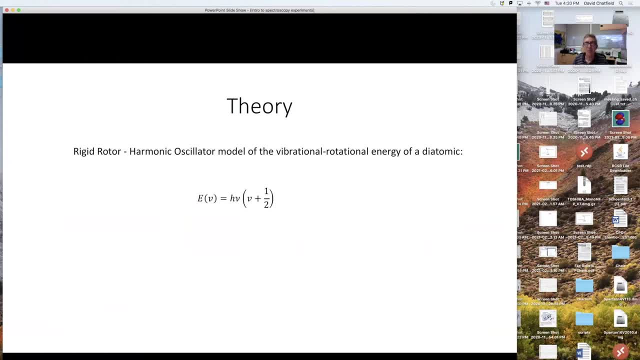 it at great length. But the theory is based initially on a molecule, of a molecule as rotating and vibrating at the same time. This is a good example. So there is a few things that we'll look at in the lab to see if that's a good example. So let's start by looking 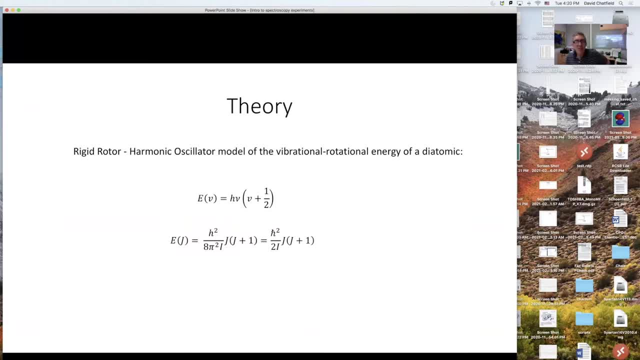 at the wasp. If you take some data like the wasp- and the wasp is potentially the most victimized material- we would observe in the laboratory- The wasp, and we also have some time. so in the simplest approximation the vibration can be thought of as a harmonic oscillator and you 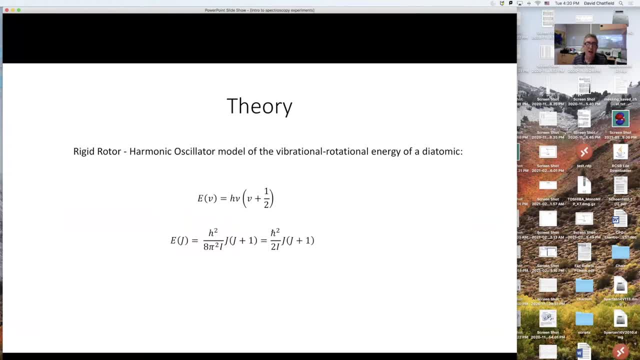 have from class, from the model problem, harmonic oscillator of the equation for the energy there, where v is a quantum number and this nu is the vibrational frequency. and then we also have for the rotation, the rigid rotor model. you can think of your molecule as now, you think of it as rigid. 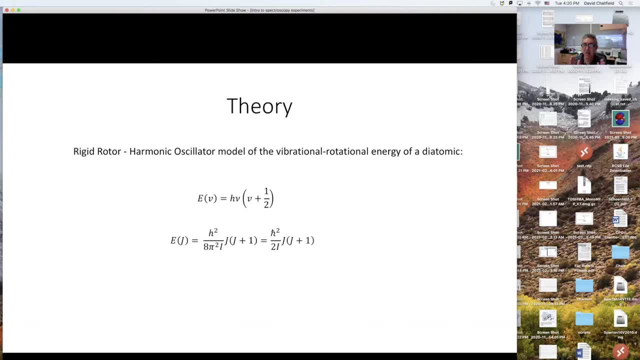 and not expanding or contracting in length. then you can have a constant moment of inertia, and this is the energy expression. it's really the same expression as you would get for a particle on the surface of a sphere. okay, it's interesting that they are analogous problems. so we have these. 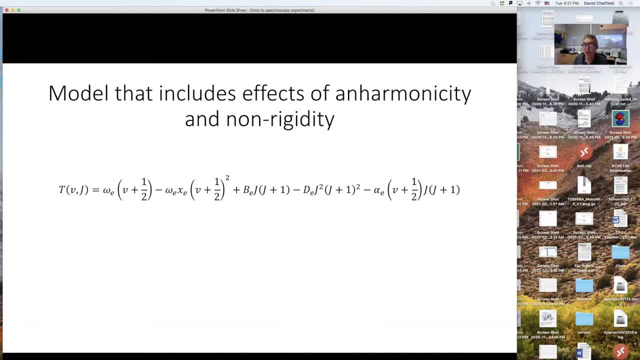 two expressions. now, real molecules are more complicated because they're not rigid and you in fact. the previous picture is not entirely consistent. right, if you're rigid you can't be vibrating, but you could individually have those two approximations to think about vibration in one. 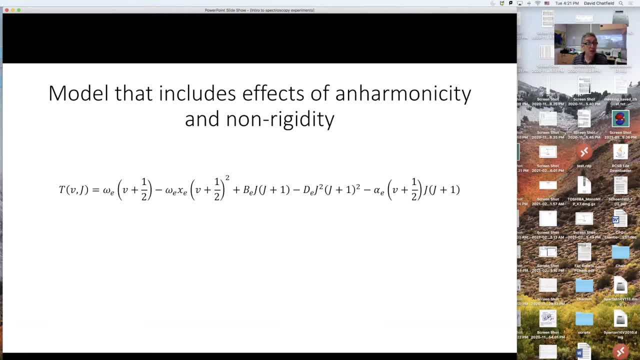 case rotation in the other. what happens when you really relax and allow for reality to set in? then the harmonic oscillator approximation has to be extended and the rigid rotor approximation has to be extended. and now we have these various terms here. first, on the left, we have our energy, except we are now expressing it in units of wave number. 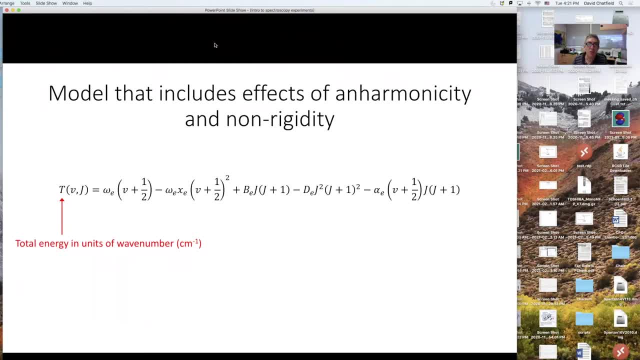 essentially, what we have done is to just divide the energy by h, c, where h is Planck's constant and c is the speed of light, and that gave us our t. the t is called a term. okay, then the next terms, using the word in a different way, on the right hand side. the first is, of course, the 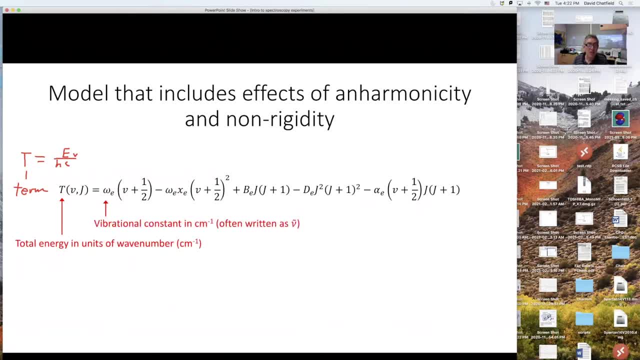 the first is, of course, the harmonic oscillator term, and omega e is the vibrational constant in class. we often use nu tilde, but here it's the omega. the next term is and queruminosity and the reflex of the kinds of overcoming, or especially of your. 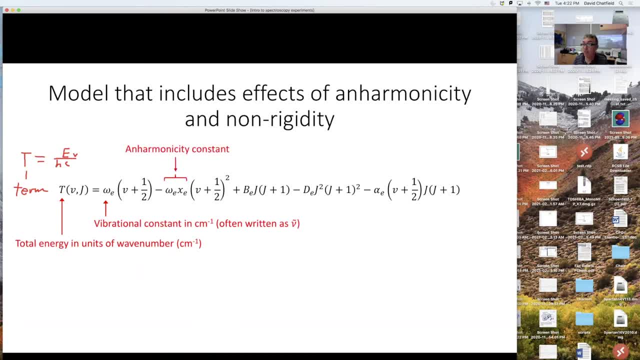 own. what can? we would put into our finaléta d, we could write a definition of what should be the different を 악. This is a correction to the harmonic term, and so the anharmonicity constant is really this double thing, this product of omega e and xe. Sometimes we call xe the anharmonicity constant. 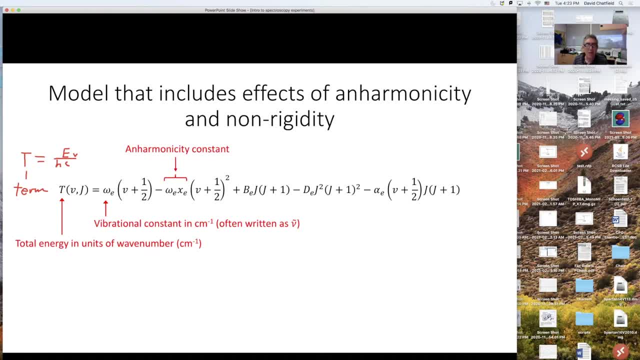 but really it's the product there multiplied by v plus a half squared. The next term is the rotational constant, a term we saw before for rigid rotor rotation and the be is the rotational constant, So it looks like what we saw before. now we divide it by hc. The next term is for: 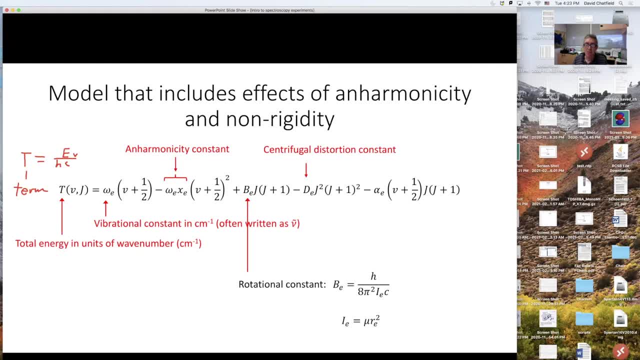 centrifugal distortion. What you have to have in your head here is: as the molecule rotates more quickly, the centrifugal force stretches it. The moment of inertia there essentially increases, and this changes the energy. It actually decreases the energy. So we have a constant that is. 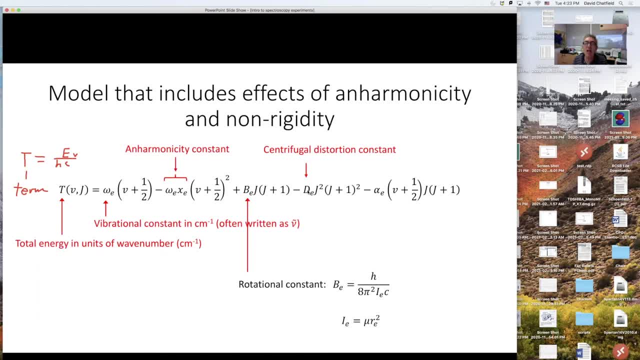 proportional. Well, the constant here is de. We make that. let that be positive, but this is a negative sign here. This is times: j, j plus one squared. so j squared, j plus one squared. Finally, there's another term, that is the coupling. describes the coupling between rotation and. 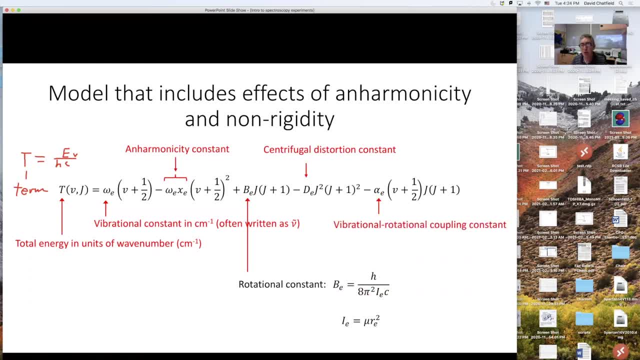 vibration, and so this is proportional to something called a vibrational rotational constant, and that's multiplied by v plus a half, j, j plus one. Okay, so you're going to use this expression to model your vibrational rotational spectrum. Okay, so now let's talk about the spectrum. 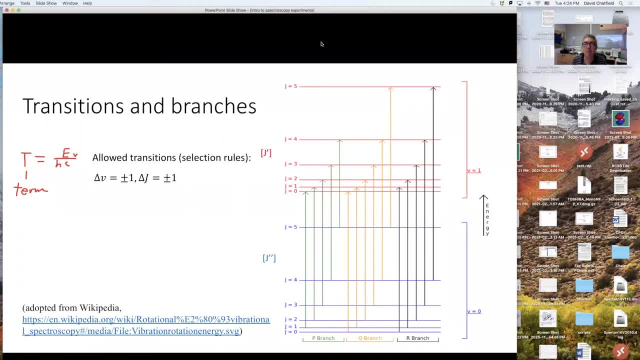 itself. Okay, so we have to talk about the transitions that we see. We have to talk about which are the allowed transitions and the selection rules. Selection rules are what tell us which are the allowed transitions and the selection rules are what tell us which are the. 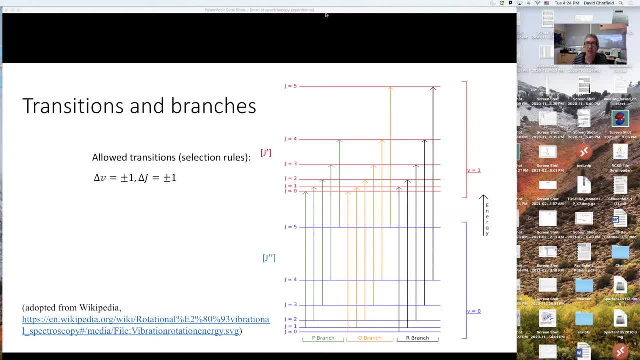 what transitions are allowed and what are not. Now, the general principle here is that we start in some initial state and your molecules in that initial state. that initial state is described by quantum numbers v and j, and we'll often use a double prime to describe the initial state. 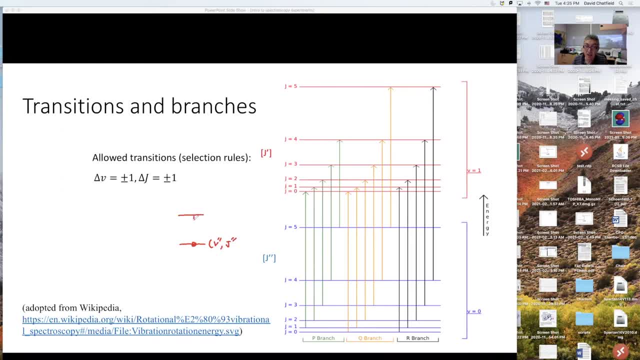 Then there's some higher energy state that we can excite. Of course we need some energy, something to excite. so the energy comes from a photon that has some particular frequency And that will excite us to some upper state described by a new value of v. 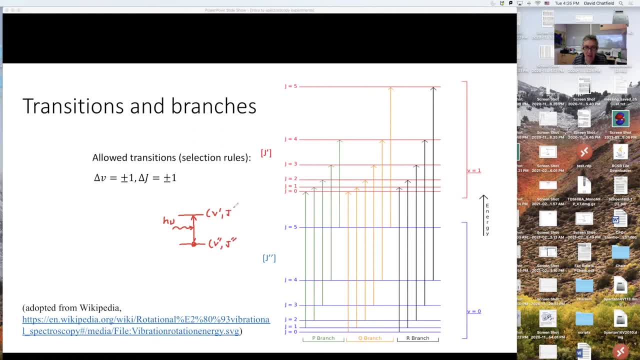 We'll call that v prime, and a new value of j, we'll call that j prime. Okay, so in blue here we have the different possible initial levels. so in every case v is equal to zero, but we have a different set of possible values of j. these are: 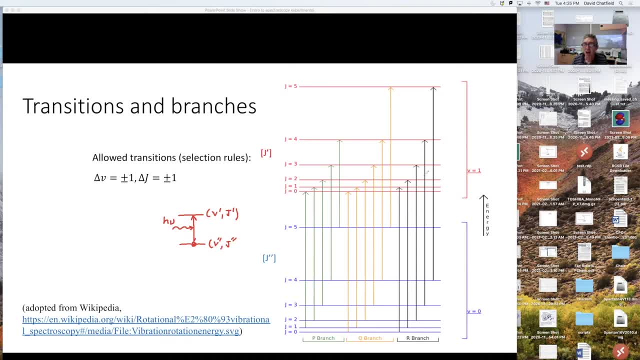 all the initial states um. up above, you can call this if you like- the v equals zero manifold, manifold of different j's um. if up above we have the unexcited state where v equals one, and again we have this manifold of different j values. so we are going to see excitation out of 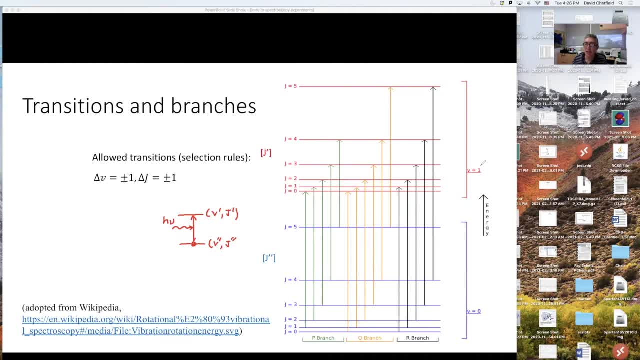 the v equals zero manifold up into the v equals one manifold, and these vertical arrows show the various transitions we might see. so let's talk about these um first. let's talk about this line we're starting in: v equals zero, j equals zero. going up to v equals zero, j equals one. okay, so. 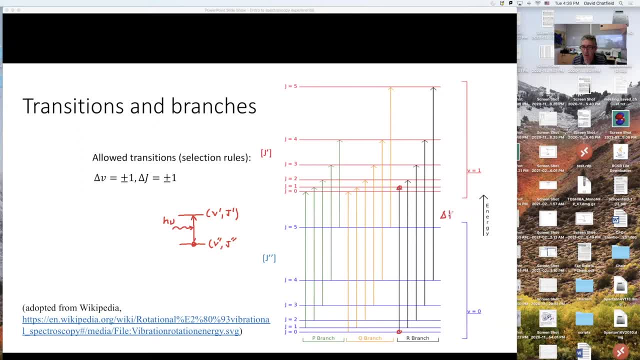 that's a delta j. okay. so that's a delta j equals plus one. transition: okay. in the next case we can go from j equals one up to j equals two. that's also delta j equals plus one, and so on. here we go from two to three and three to four. 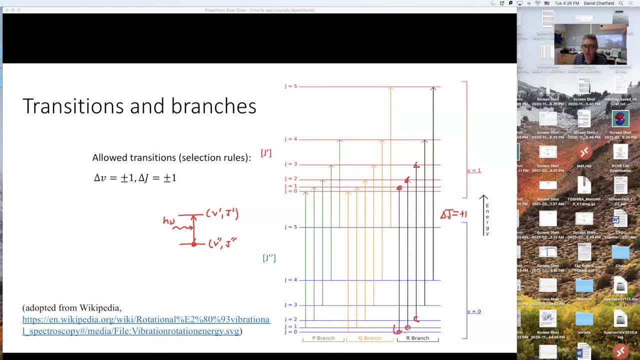 so all of these together right here are for delta, j equals plus one, and we call this a branch, the r branch. okay, now over here in green notice, here we're going to name from j equals one, v equals zero, j equals one to v equals one, j equals zero. 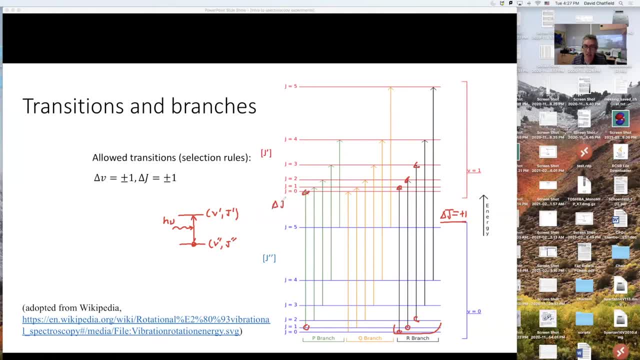 so this is delta j equals negative one. here we have j equals two, going up to j equals one. again, delta j equals negative one, and so on three to two, etc. so this delta j equals negative one. branch we call the p branch right here and in. that's all you're going to see. For some molecules delta J equals zero is allowed. 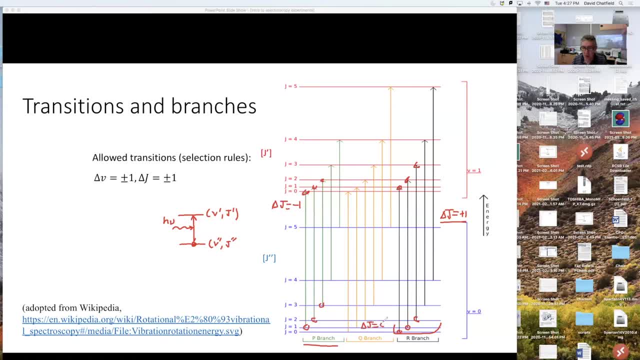 So when delta J equals zero, we talk about a Q branch. However, we don't see the Q branch. It's forbidden for HCl. And why is it forbidden You'll see later in the class. Okay, so every peak that you see in your spectrum comes from either one of these. 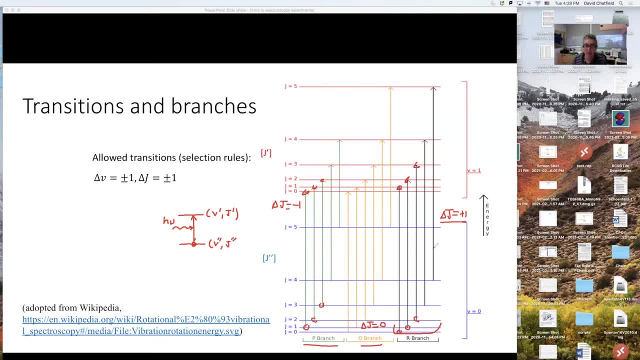 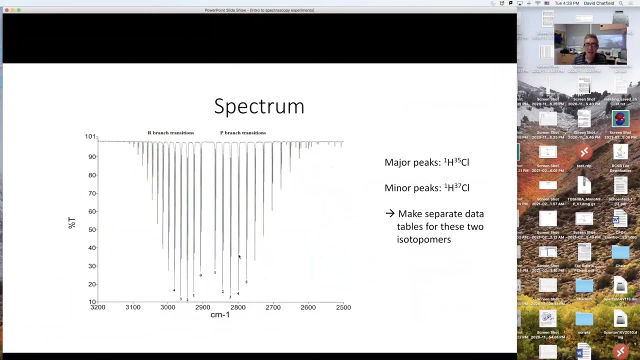 blue or one of these, one of these green or one of these blue or black, I guess they're black transitions. Okay, moving along better. So your spectrum. So you'll get the spectrum and you will label it. You can label it down here. 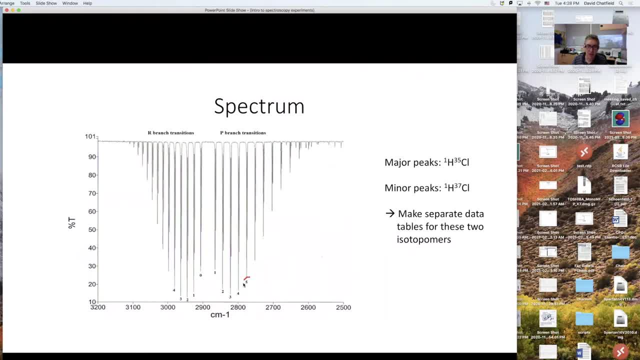 It's labeled by the value of J double prime, right, Right. So for the P branch the smallest value of J in the lower state was one. In the R branch, zero was allowed. So these are labeled by J double prime. 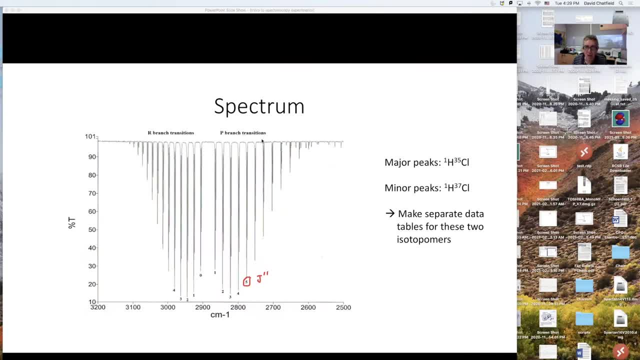 So P branch and R branch. Now you'll also notice, if you look closely, that every peak is really a double peak, And I'll focus on this one. for example, right here this peak, You notice there's a tall peak but there's also a smaller peak. Okay, that's because chlorine has 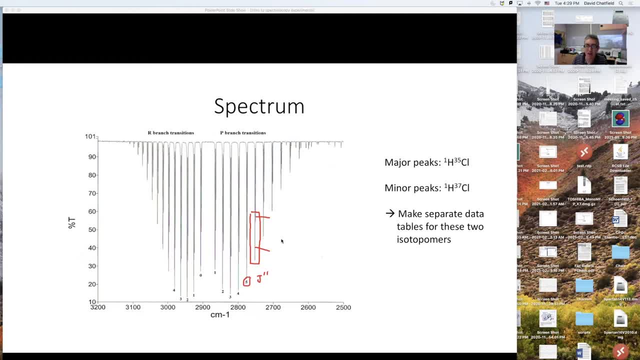 a fairly common isotopes: 35 and 37. So this tall peak. it turns out that 35 is more abundant, So this is H135Cl and the other one is the H135Cl37.. Okay, of course we speak of isotopes when we 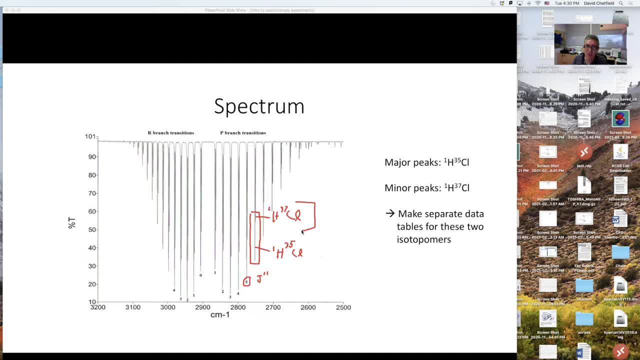 speak of atoms, but when we speak of molecules- that's that's our composed of individual isotopes- We use a different word: isotopomer. right? So these are the two most common isotopomers of HCl. Okay, So you'll label. 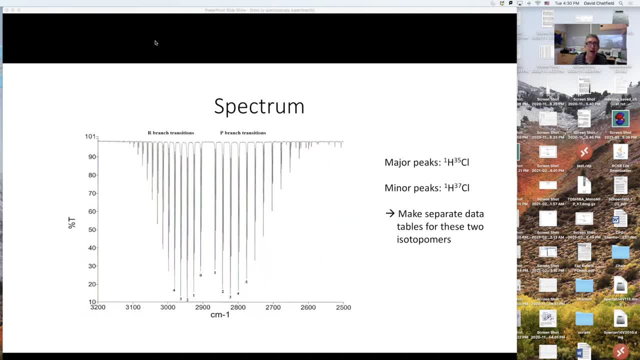 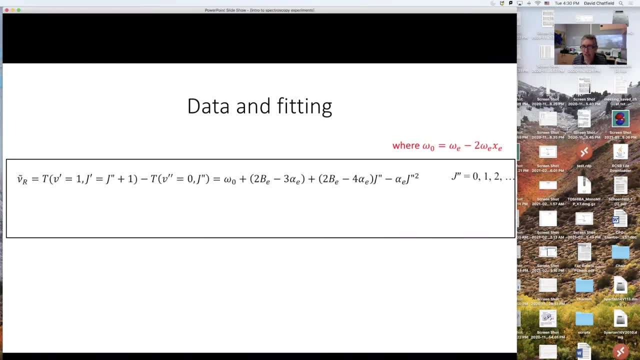 your spectrum this way and then you'll analyze it. How do we analyze it? Let's go on to the next slide So you'll fit your data and without going through the algebra, real fast. I've you know any slowness. you can look at the lab manual and see how to do it. 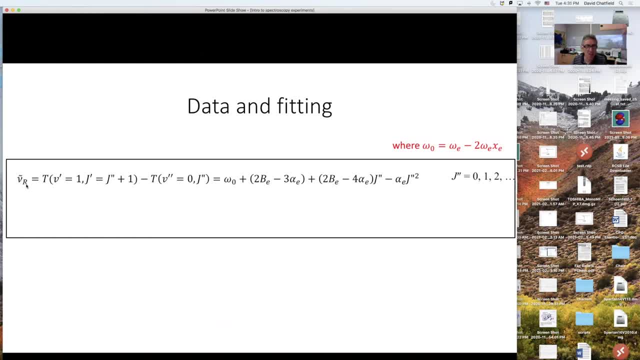 We'll call new tilde here for the R branch. Those are: the new tilde is the frequency of the peak in the spectrum. And the peak in the spectrum comes from the difference between the two energies, the upper state and the lower state energy. So that would be T for. 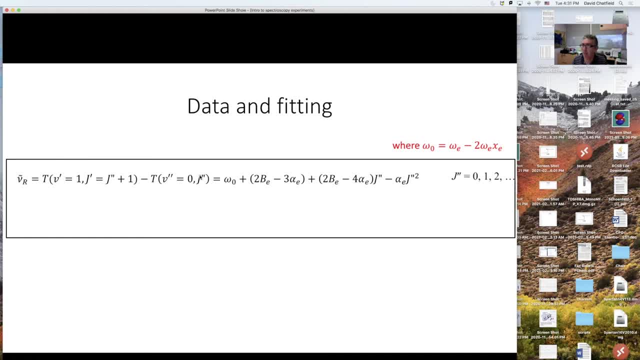 v prime, j prime minus T. for v double prime, j double prime, That's the lower state, and so when you do some algebra, this is what you get, an expression in terms of omega naught, b, e, alpha e and so forth. now, omega naught is the difference between this, difference that you can. 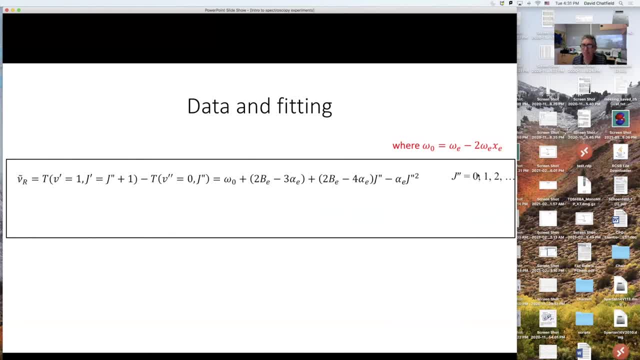 see omega e minus two omega e, x e. okay, so there you go for the p branch. you get an analogous expression. it's just a little simpler. okay, now, we in this expression we have not included the centrifugal distortion. we can do that also, but we haven't done it here. now you can combine. 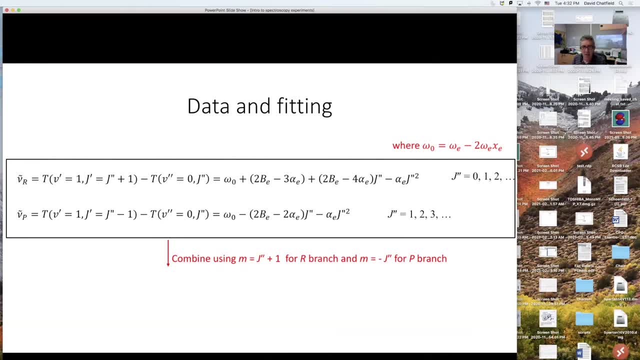 these two expressions, as is described by, just by defining m as j double prime, plus one for the r branch and minus j double prime for the p branch, you get this, this expression in the quadratic fit, this expression for the cubic fit. you might as well just do a cubic fit your, your resolution. 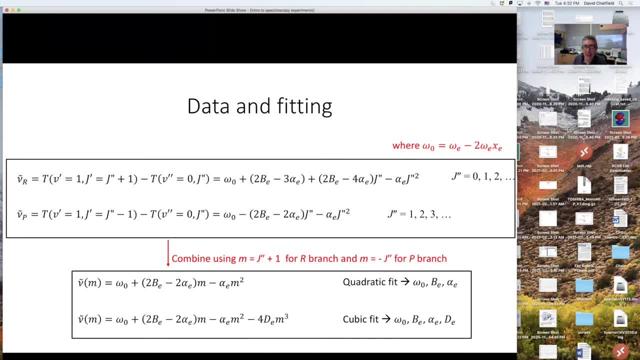 is high enough that you can get a value for d e. that's meaningful. if you didn't have such high resolution, there'd be a lot of noise and you shouldn't try to get it. but you can get it, okay, so you will then fit all of. 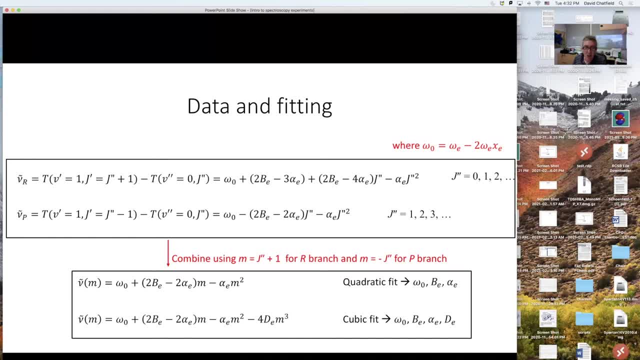 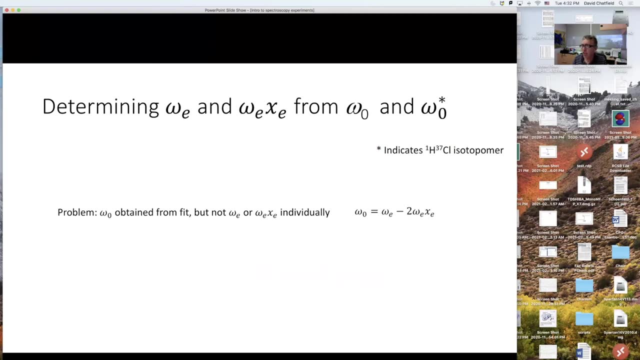 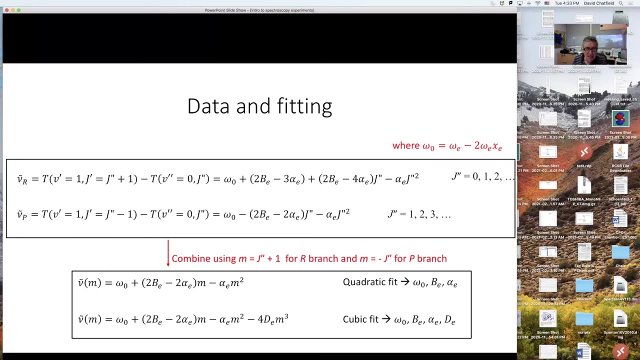 the lines in your spectrum using a cubic fit. you can do this in excel using a trend line, with a polynomial trend line in third order, and you'll be able to obtain all of your, all of your constants. now one additional note. if i go back, actually, you'll notice what you can get out of this fit is omega zero. 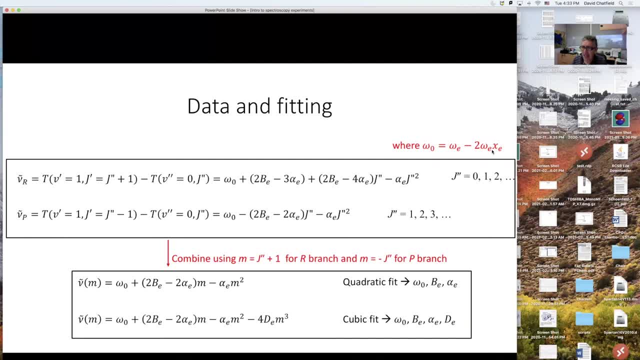 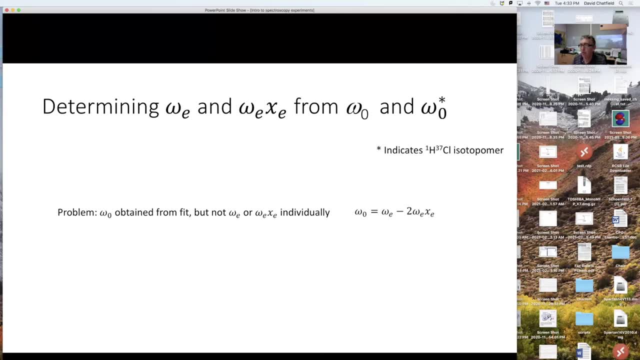 but you'd like omega e and omega e xe. how do you get them? well, you can get them by combining the data from the two isotopomers. okay, so for i, one isotopomer, we have this definition of omega naught, and when we get to the second one, we get the definition of omega naught. 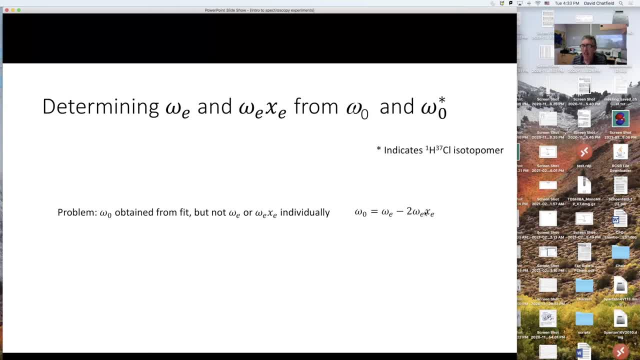 and when we get to the third one, we get the definition of omega naught, we have no asterisk. we'll be describing, uh, the 31h35 cl isotopomer. so for the other isotopomer, um, we have of course this expression where the asterisk just means. 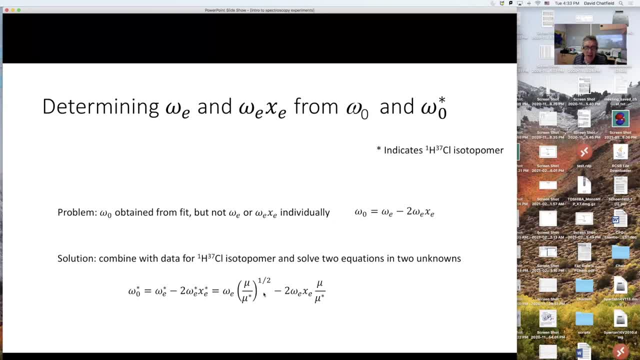 37, um, and you can do a little algebra and get this. now, where does this come from? um. let me tell you where this comes from. remember that um, omega e is the square root of the force constant divided by the reduced mass. now, if that's true, then omega e- asterisk. 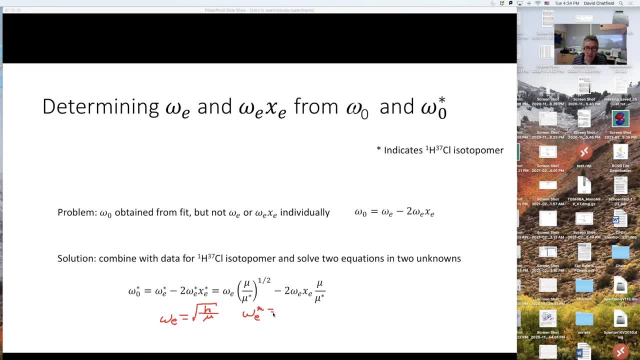 will be k divided by the reduced mass of the 37 cl isotopomer. that's that asterisk here. now k, the force constant, is going to be the same in both cases, but the reduced mass is different. so you can do a little algebra and write this as: 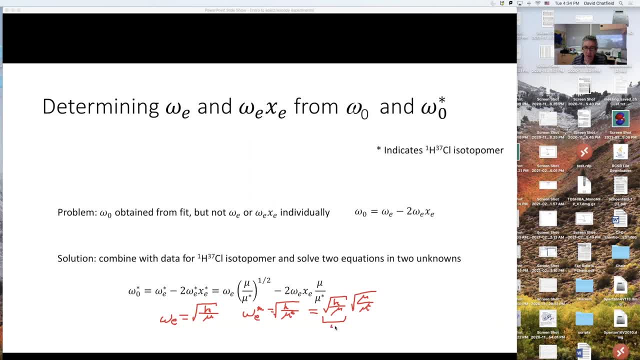 and of course, this right here is just omega e. so that's, that's how you get this expression up in right here. and then, once you've got that notice, you have two equations and two unknowns. here's one equation, because this is not an unknown, that's measured from your spectrum, and here's the other other equation. 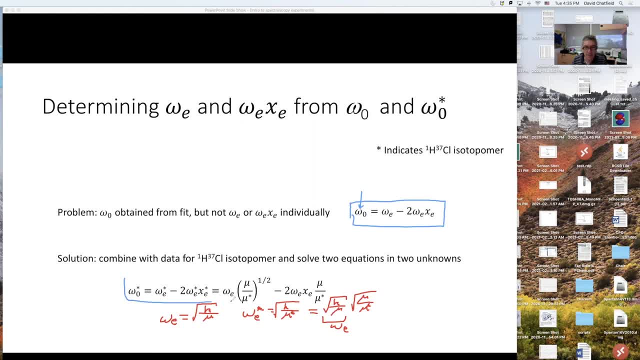 right here. so if you look at this equation, this is a oh, so you have the those ones here. you can come up with these points, right kinds, and then to certain parts, and then make us more equal, and so that's the answer to that. the third equation isều. so our unknowns are what i'm going to circle, omega e and omega x, e. so we have two equations, two unknowns, and we can determine both omega and omega y and we'll be divided by the unknown. so omega and y, all the other equations, in particular Jeff, we cure as best we fool around or be able to solve the result in something that says omega e and omega y are all wrong. so we can deal with this and we'll consider omega fields, although the music speaks of the. so and if our, our relationship entity manually works well, and in fact this is why we can.